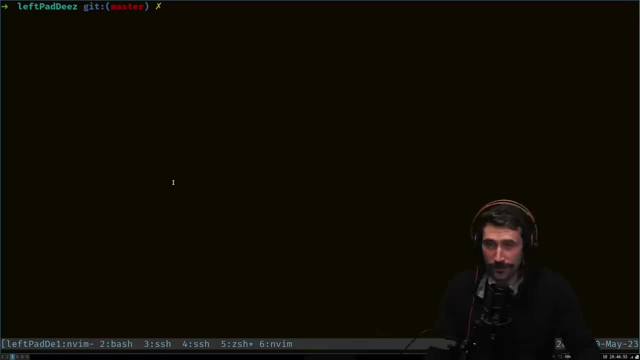 But why? Well, first off, you're probably running them on your computer, Which, if I just go pgrep node, I don't even know how I have that Dude. I must have a Bitcoin miner on my machine. I do have Zig running. 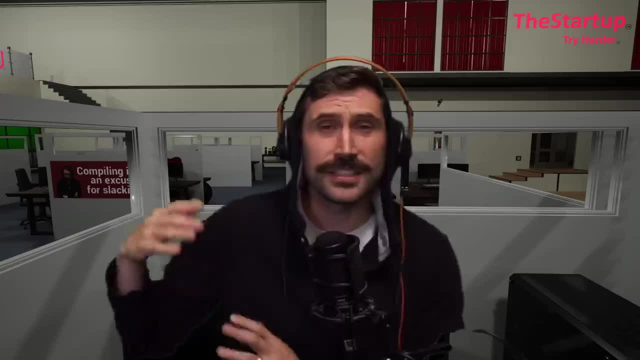 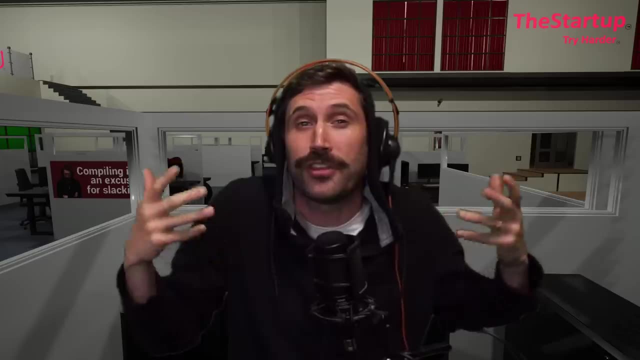 Hey, calm down, ladies and Arch users. okay, I'm taken. Tests also often hide implementation details, such as garbage collection. When you run these micro benchmarks, they don't necessarily trigger all the things that could happen when you're running in production. And finally, it depends on what you're actually doing in your function. The thing about JavaScript is that strings aren't strings, They're actually rope Data structures And there's a lot of optimizations around concatenation and appending with a heavier penalization of iterating over each character. 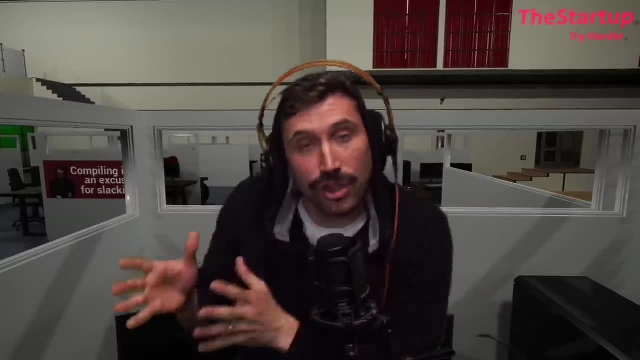 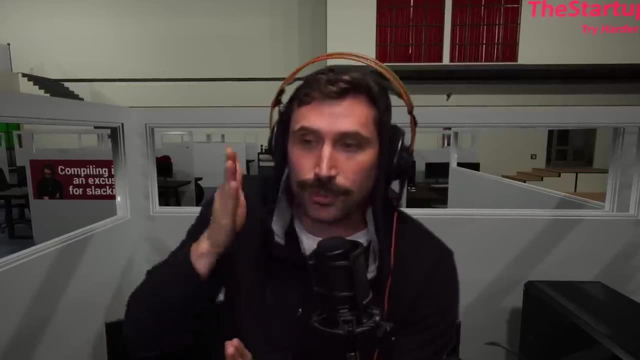 So that means if we're just appending a bunch of strings together, it may look good on paper, But when you actually use the string to do something- say send it across the Internet or print it out- it has to iterate over a more complicated structure to get that string back out. 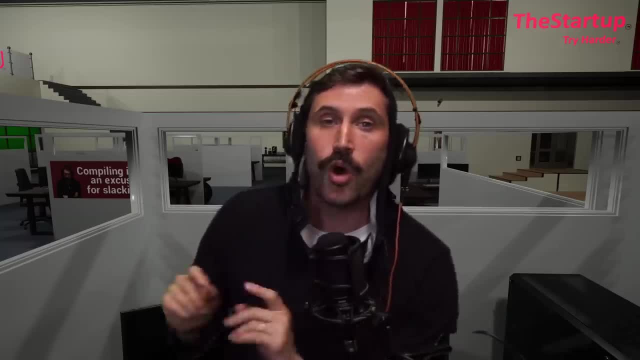 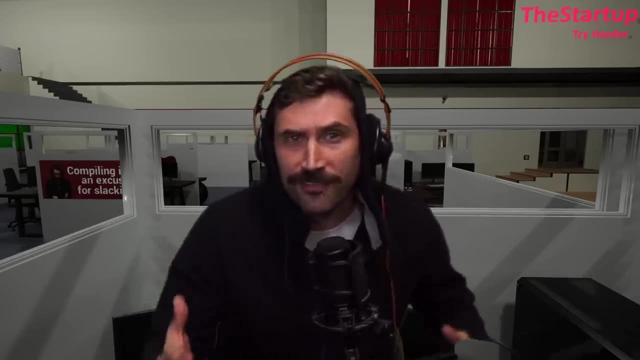 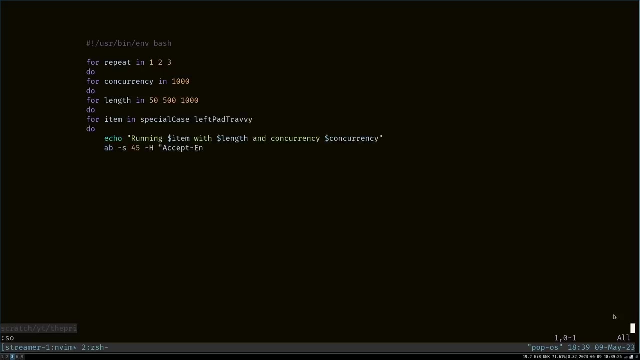 So you pay none of the cost of using your string. You only pay the cost of producing it, which could be cheaper, thus giving you misleading results. So how do we determine which left pad is actually faster? Well, first I created a server, set up Apache benchmark script and ensure proper sleep between each, and manually execute garbage collection on the server if no requests have happened within one second. 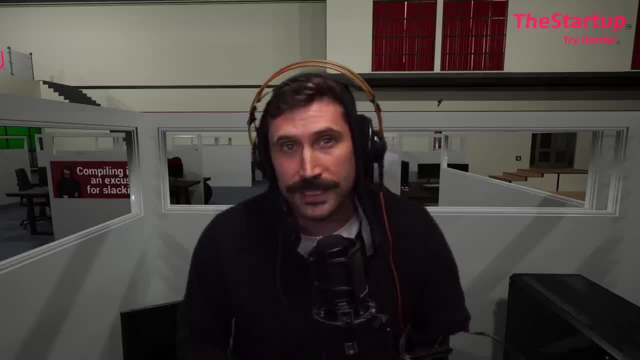 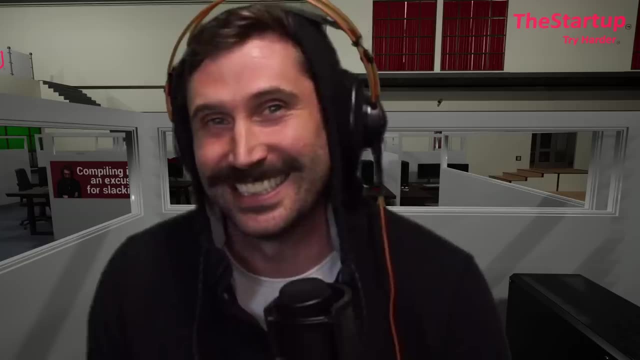 Sent 50 million requests that took about 36 hours to complete. I'd personally like to thank Linode for giving me an instance to run this on and not shutting me down after 50 million requests. Thanks, Andrew. Create a parser to parse the Apache benchmark results and calculate the average of media. 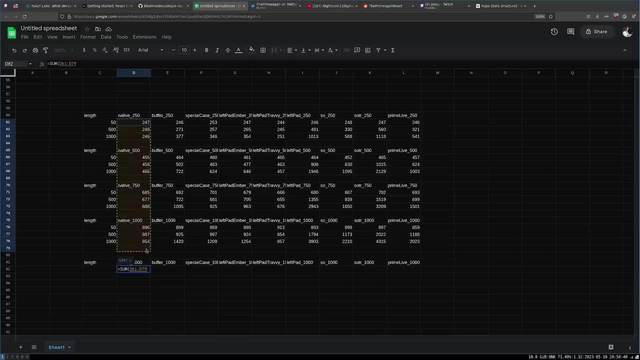 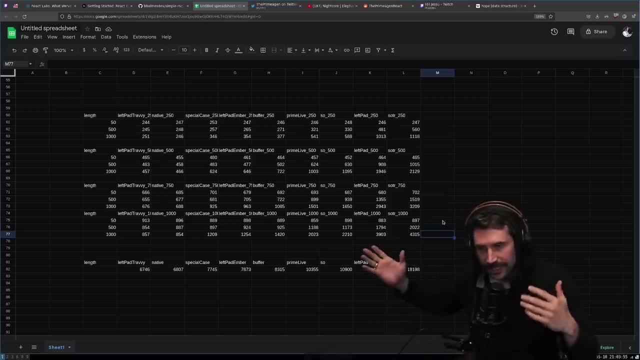 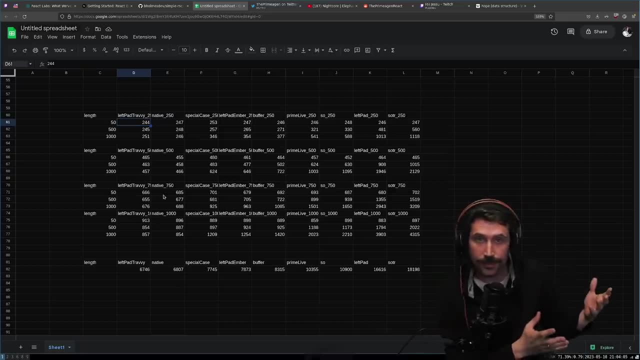 Charts. Before we dive into the charts, let me explain what the data is you're looking at. So each one of these points is the average of the median. So what I did is I do 12,500 requests and I take the median time of that. 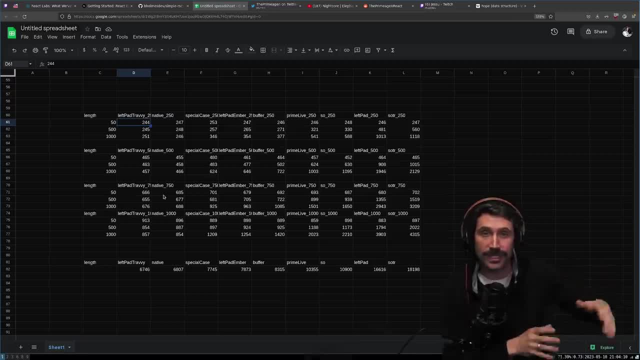 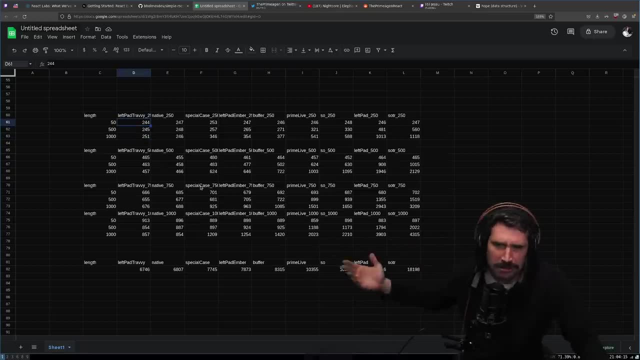 And then I do it again, and I do it again, and I do it again, And after a bunch of those requests I'd have several amount of medians, and then I take the average of those. So each one of these represents somewhere between 50,000 to 100,000 requests each. 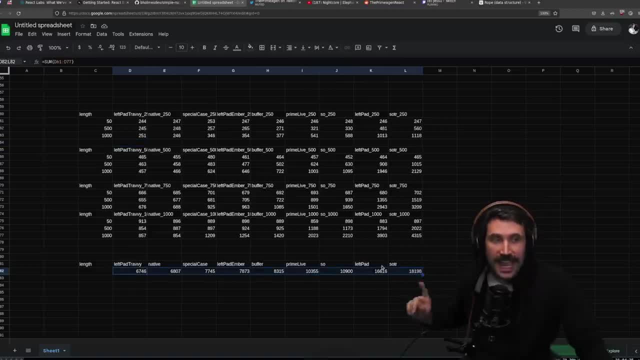 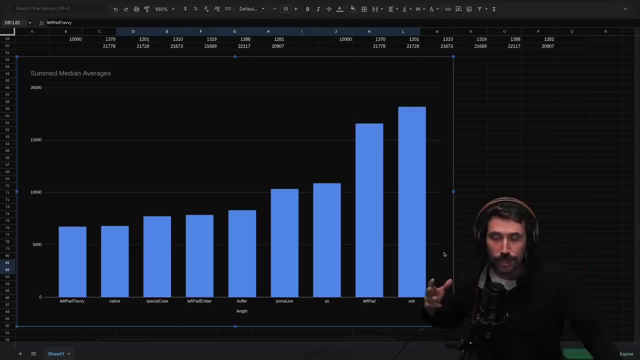 And then, of course, down here, I just simply summed all those numbers across every size of request, and then i ordered these columns according to who had the largest sum. all right, so this chart's probably the most important chart to look at is the summed. 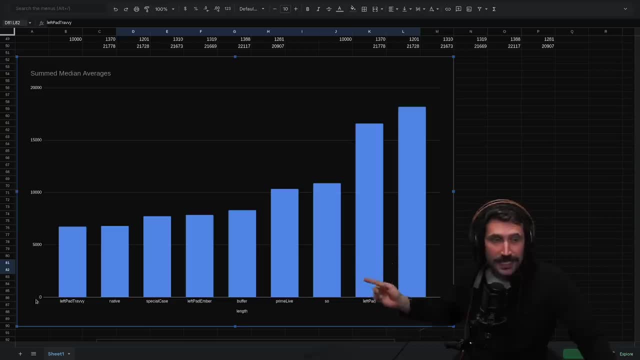 of the median averages. on the y-axis we have milliseconds and on the x-axis we have the different left pad summed averages of the medians. so worst place came in as the stack overflow tail recursive version, which i'm a bit surprised by. then came left pad commanding a strong. 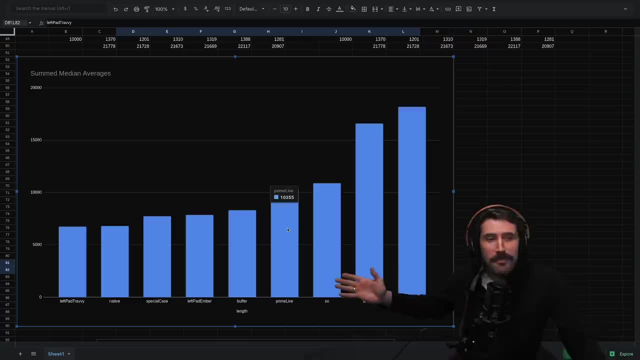 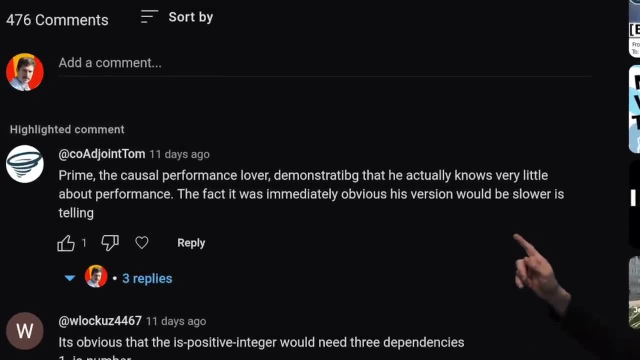 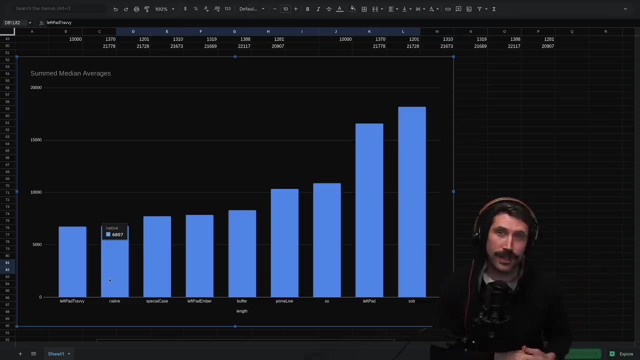 second worst place. then look at this. my version was faster, okay. so after all of the jokes and the mean youtube comments, i'm talking about you, tom. it hurt, but the fastest really came down to left pad, travi and native. they're really within a margin of error of each other. so what is the 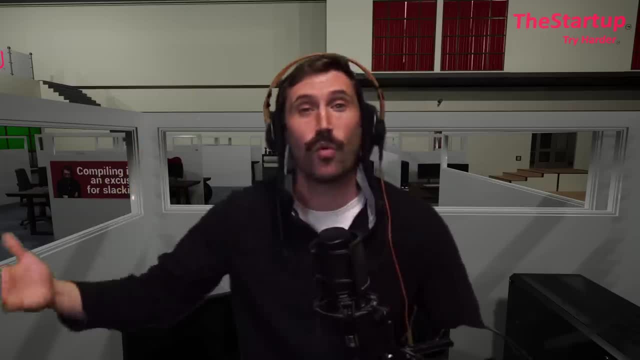 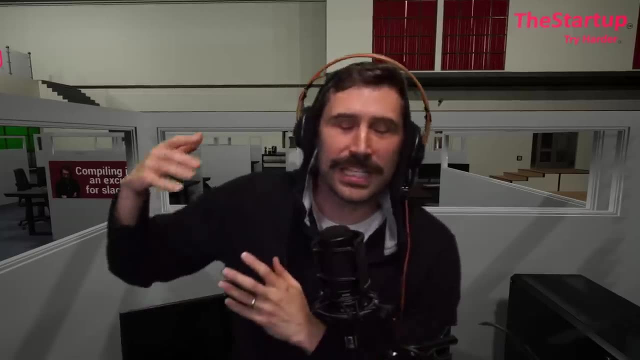 takeaway of this? the takeaway is: use native methods. they're way better. you don't have to be clever. you don't have to write code that looks like that, whatever. then what is this? and the best part is, you don't have to be clever. you don't have to be clever. you don't have to be clever. 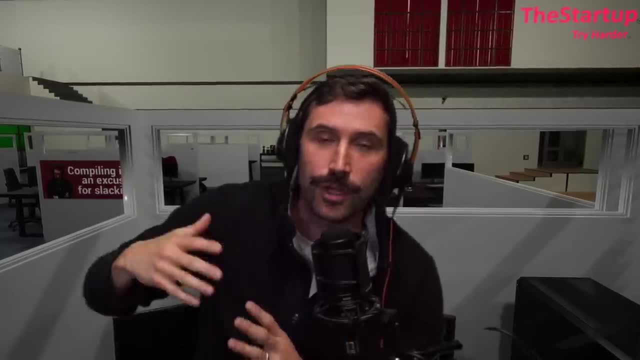 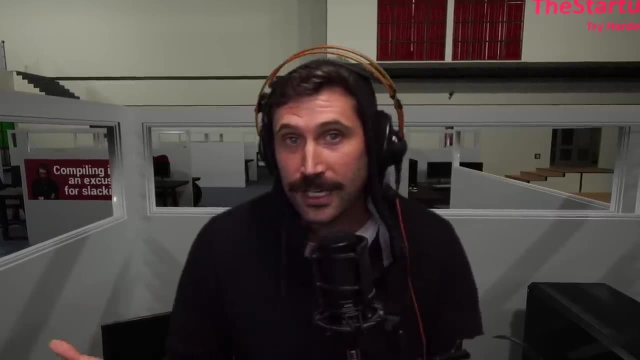 is is that as new techniques come out, as things happen over time, you don't have to make these weird changes to your code, where you did these weird incantations to figure out what code's actually faster than the other code. instead, you know, the platform is motivated to make a fast. 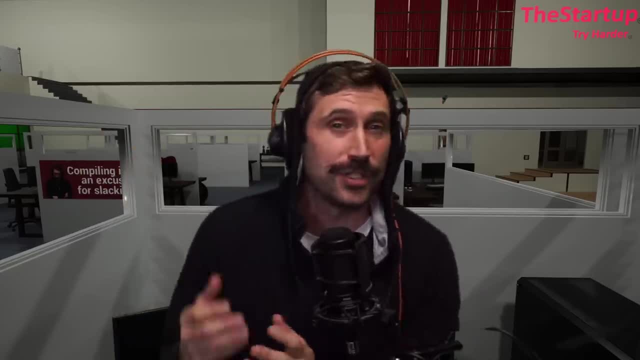 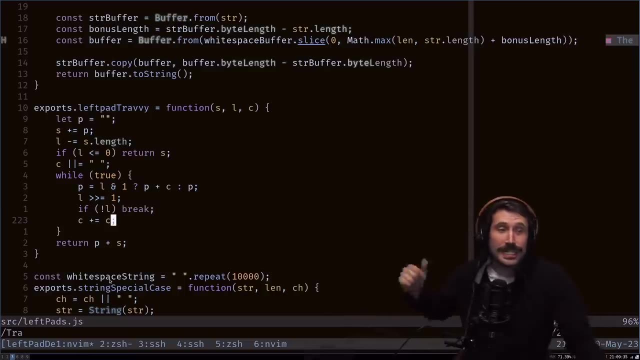 product. so stick with syntax or vendor implemented options where possible and you will mostly get the best performance. but if you ever feel spicy and you want to do power of two, string concatenation and bit shifting, well, go ahead, give it a try. which is funny because that's actually how. 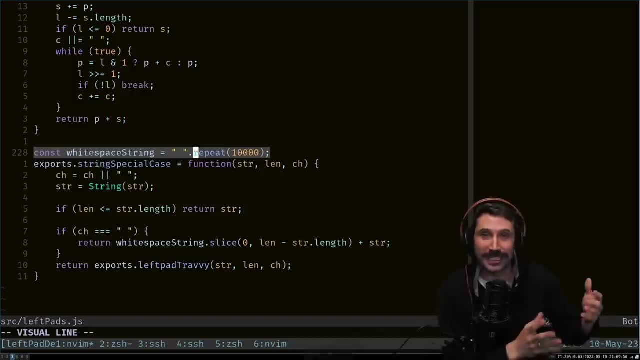 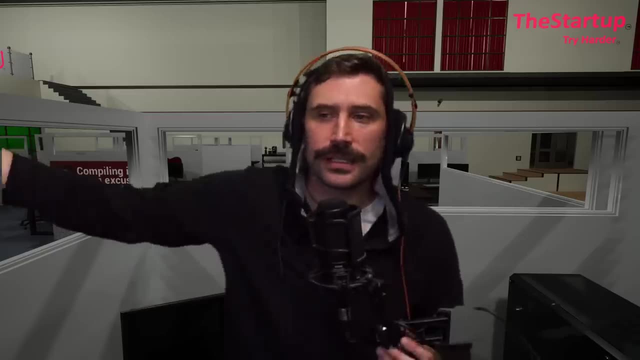 stringrepeat works is power of two string concatenation and bit shifting in v8. i don't, i don't, i have no idea why that's fast. i literally have no idea. hey, if you like this, press the like button, press subscribe. come on, give me some signals. okay, if you want more of this, send me. 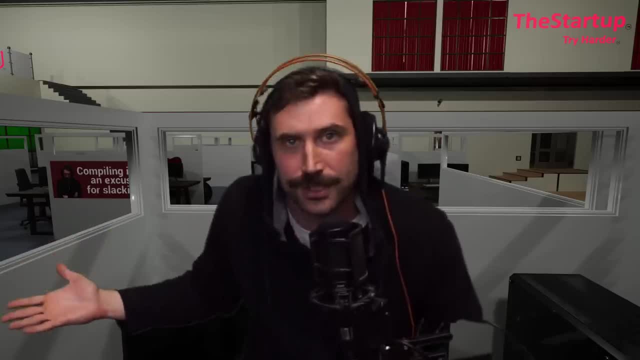 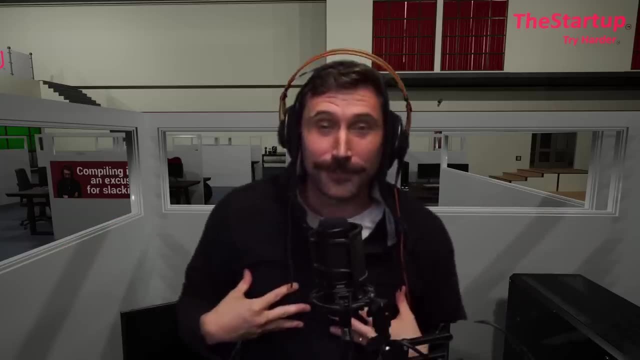 the signals, make comments, do all the stupid things you know you're supposed to do already. okay, because youtube highly favors that. so if you don't do it, it makes me feel like this is a failure. and then i feel like a failure and then my wife thinks i'm a failure. don't do it to the wife again. this is for you, travi.